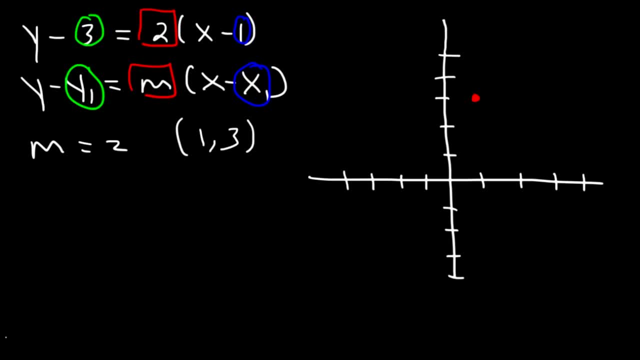 That means, as you travel one unit to the right, you need to go up two units. So the next point is going to be at 2, 5.. So if you go 1 to the left, you need to go down two units. 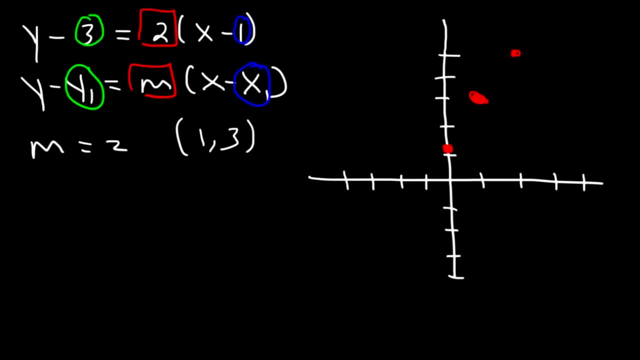 Now, granted, this line is not going to be perfectly straight, but you get the picture And then just connect them with a straight line. Let's try another example. So let's say, if we have this equation: y plus 3 is equal to 3 over 2 times x plus 4.. 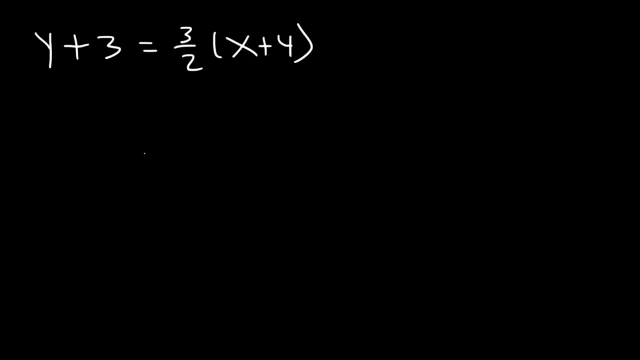 So identify the slope and the point. We can see that the slope is equal to 3 over 2.. Now what's x1 and what's y1?? x1 is negative, 4, y1 is negative 3.. Basically, you just got to change the sign of these numbers. 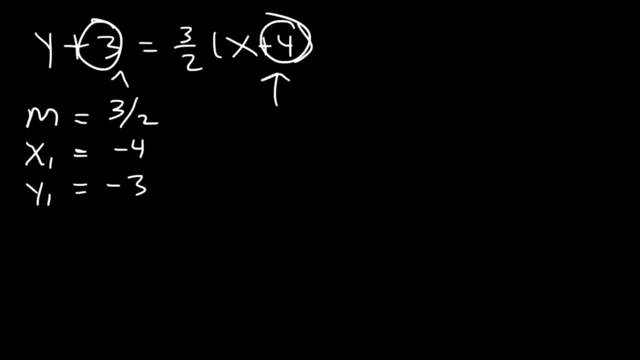 If you see a plus 4,, make it a negative 4.. If you see a positive, 3,, make it a negative 3.. If you see a negative, 3, make it a positive 3.. If you see a negative 3, make it a positive 3.. 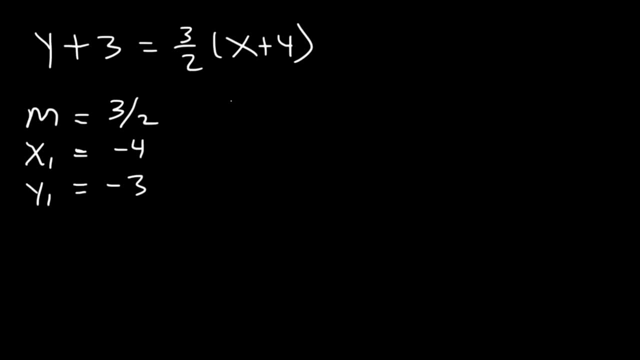 So just reverse the signs and you're going to get the point which is negative 4, negative 3.. So now we can go ahead and plot it. The first point is at negative 4, negative 3.. And the slope is 3 over 2.. 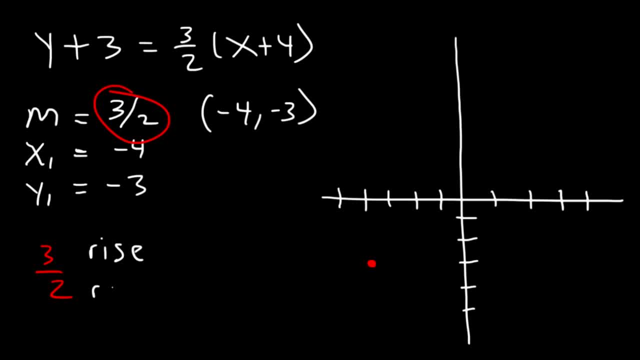 3 is the rise, 2 is the run. So we're going to travel 2 units to the right and we're going to go up 3 units. So the next point that we're going to get is negative 2, 0.. 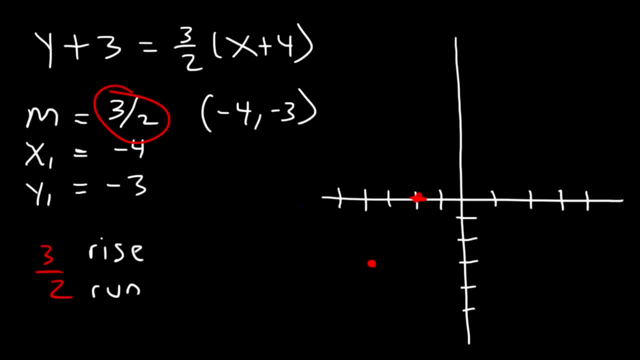 x is negative, 2, y is 0. So now let's use the slope again, Let's travel 2 units to the right and let's go up 3 units. So this will take us to the point 0, comma 3, which is a y-intercept of 3.. 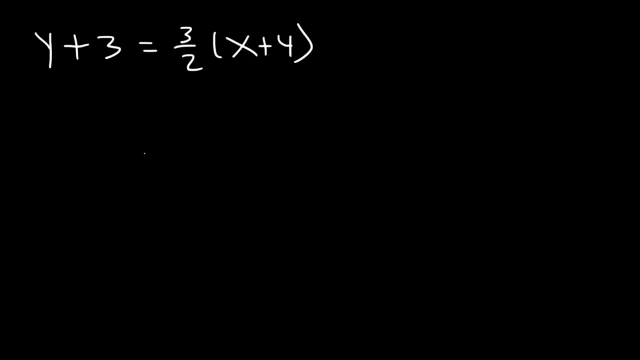 So identify the slope and the point. We can see that the slope is equal to 3 over 2.. Now what's x1 and what's y1?? x1 is negative, 4, y1 is negative 3.. Basically, you just got to change the sign of these numbers. 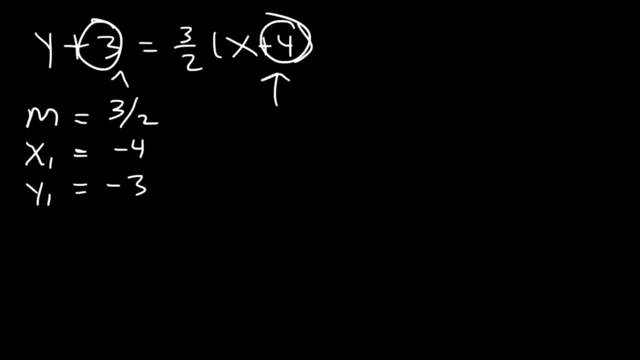 If you see a plus 4,, make it a negative 4.. If you see a positive, 3,, make it a negative 3.. If you see a negative, 3, make it a positive 3.. If you see a negative 3, make it a positive 3.. 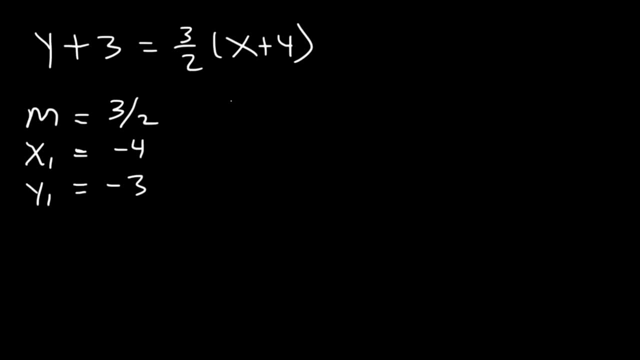 So just reverse the signs and you're going to get the point which is negative 4, negative 3.. So now we can go ahead and plot it. The first point is at negative 4, negative 3.. And the slope is 3 over 2.. 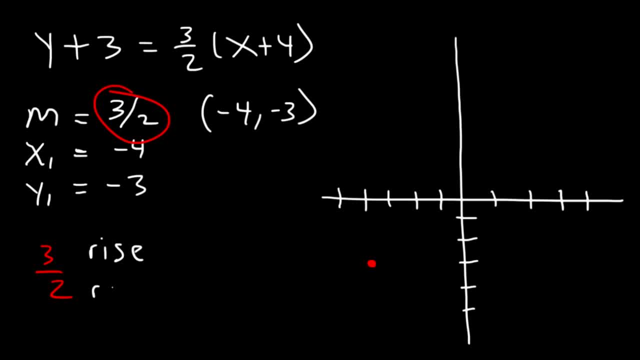 3 is the rise, 2 is the run. So we're going to travel 2 units to the right and we're going to go up 3 units. So the next point that we're going to get is negative 2, 0.. 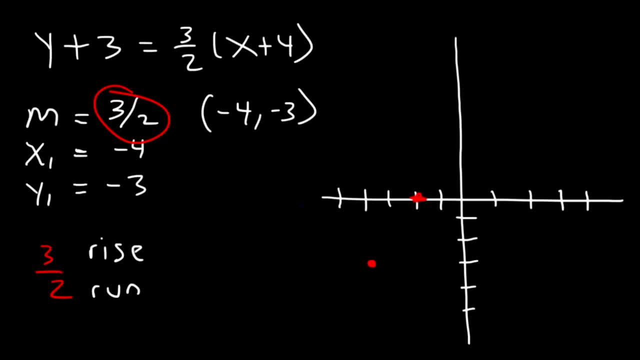 x is negative, 2, y is 0. So now let's use the slope again, Let's travel 2 units to the right and let's go up 3 units, So this will take us to the point 0, 3.. 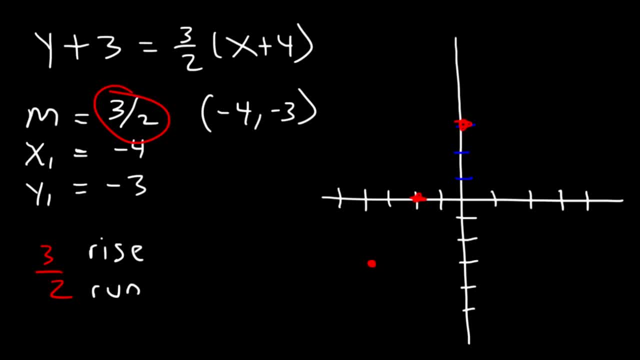 Which is a y-intercept of 3.. And now let's connect these points. So now you know how to graph a linear equation in point-slope form. So all you need to do is find the x and y values of the point, the first point they need to plot. 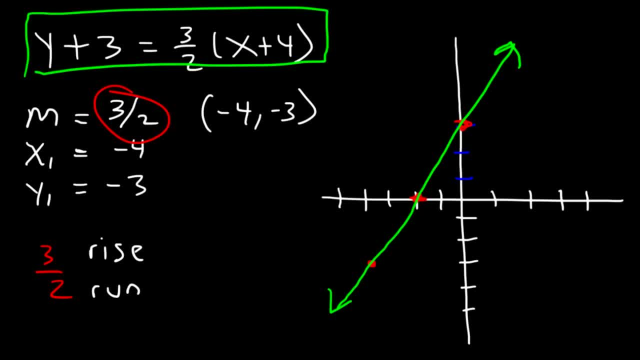 and then use the slope to get the next point. All you need is 2 points. If you have 2 points, you can draw a straight line. If you want the third point, that's fine too, but you just need 2 points at minimum to graph a straight line.